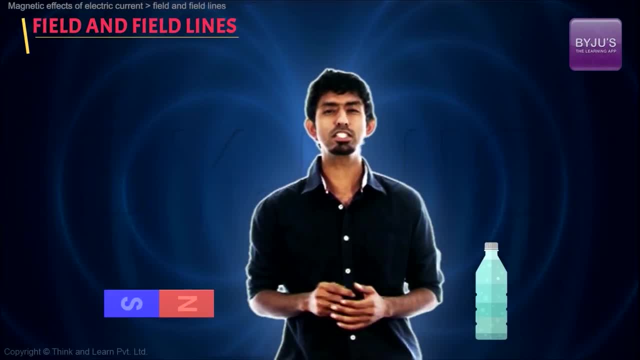 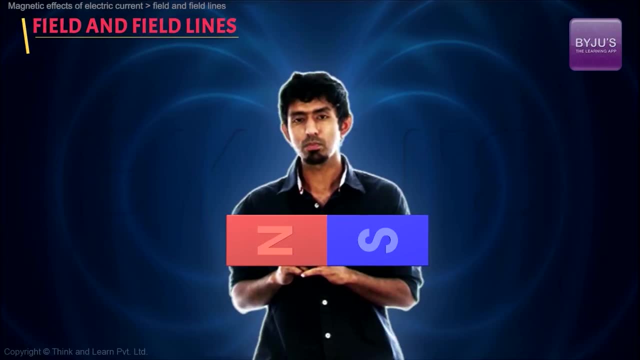 So we all know what magnets are and what magnets are not. Now let us take something like a bar magnet. What's this bar magnet? It's a very special case of a of a magnet. It's in the shape of a bar, and what is interesting about it? if you were to suspend it right from a wire, let's say such that. 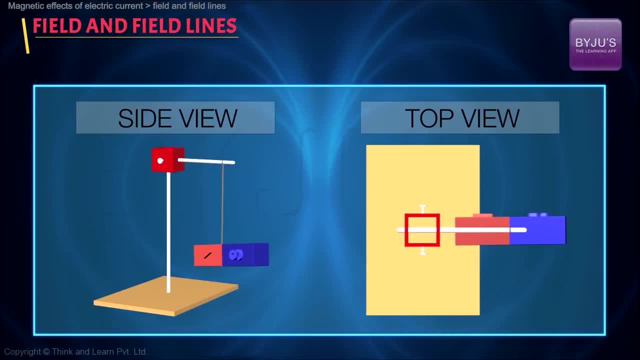 it can rotate freely very easily. then one side of it will always point towards the north and the other side will always point towards the south, very approximately. Now. why is that interesting? because even if you turn it around and leave it, it'll somehow go back to that shape itself, or 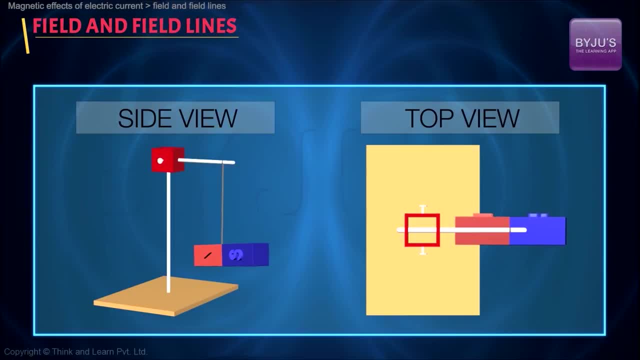 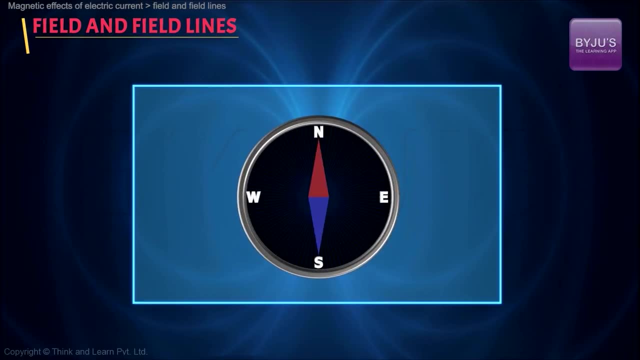 that direction itself. Why exactly does this happen? You'd have already noticed it's in one way behaving like an already known object. and what is that? A compass. So it's behaving like a big compass. so we somehow understand that if you take this bar magnet right, and even if you keep 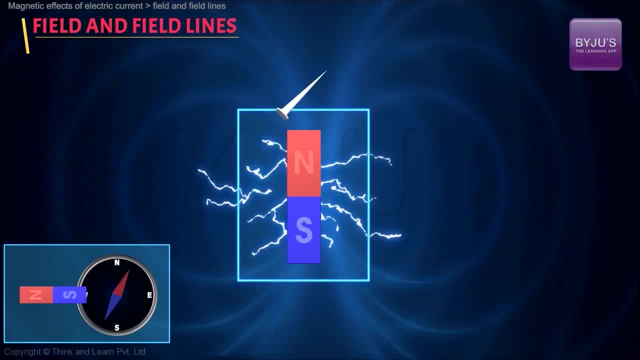 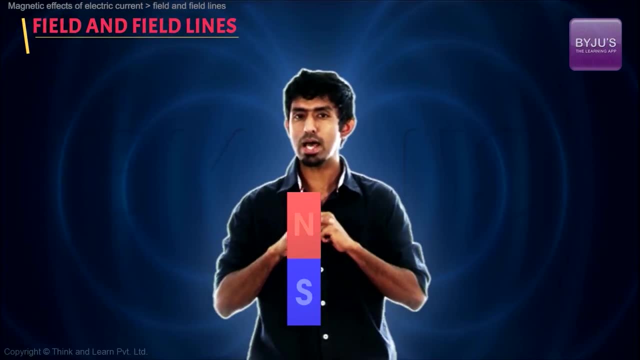 some compass near it. the compass starts to turn right. you take another little iron piece. it starts getting attracted towards it. some other small magnet gets repelled. So what we know now is that this bar magnet has some influence around it. around its area it's creating something. 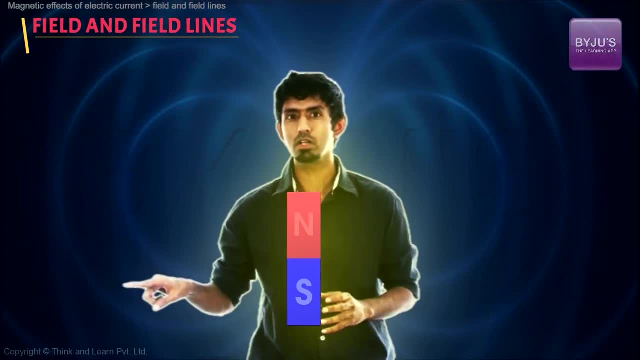 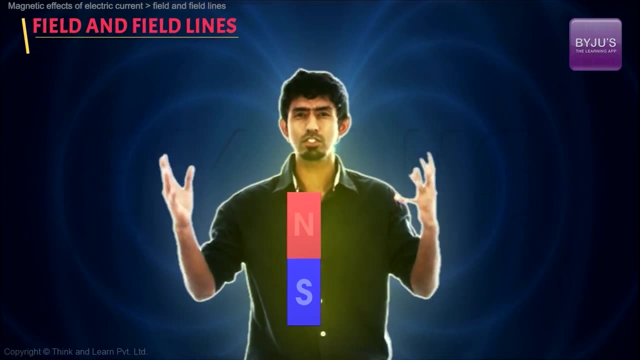 Be deceiving. know what it is, but we know it's doing something because otherwise the magnet wouldn't turn or some other object wouldn't get attracted or repelled. so now, how exactly do we look at this influence or how could we imagine this? let's do something very interesting. let us take this bar magnet put 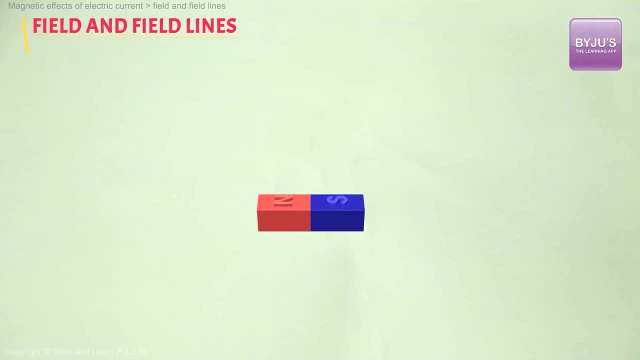 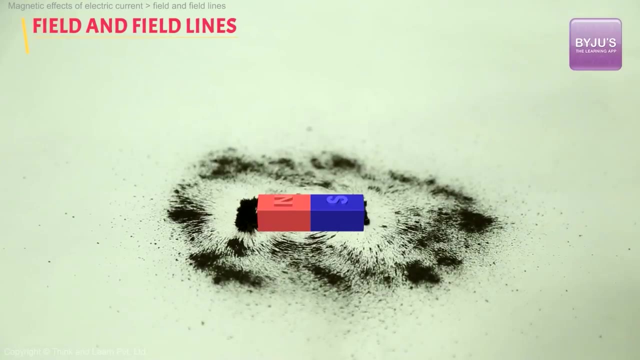 on a piece of paper right, and on that piece of paper let's sprinkle what are called iron filings. these little pieces of iron, which are like iron, is very useful for this purpose, because iron gets very strongly attracted to magnets, the magnetic substance. so you take little, little pieces of iron. 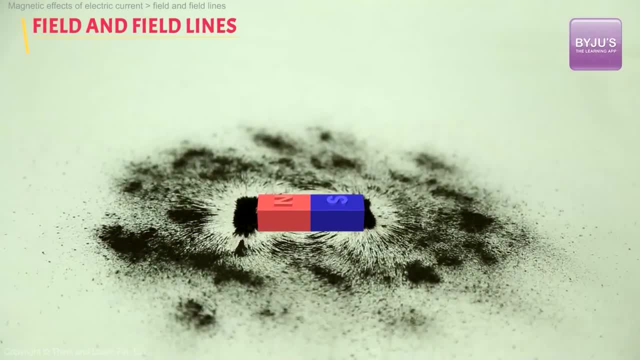 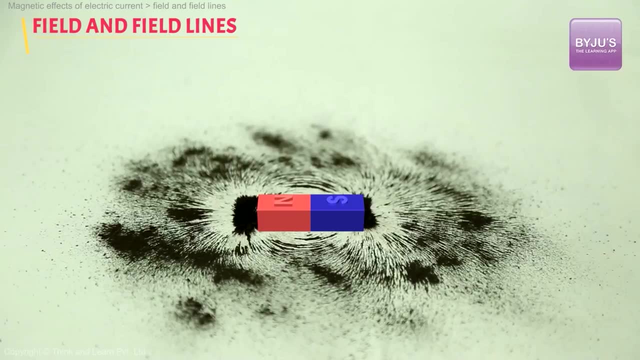 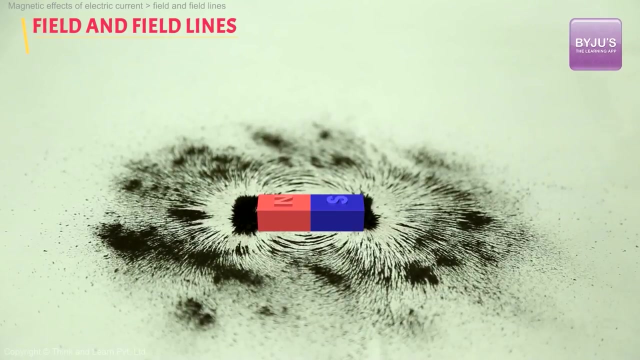 and sprinkle it all across the paper right and now gently begin to tap the paper and you start observing something really fascinating. you'll start observing that these little iron filings start to arrange themselves in a very, very, not so random pattern, in a pattern that looks like a beautifully hand-drawn thing, like what you see now. isn't that fascinating? why exactly is? 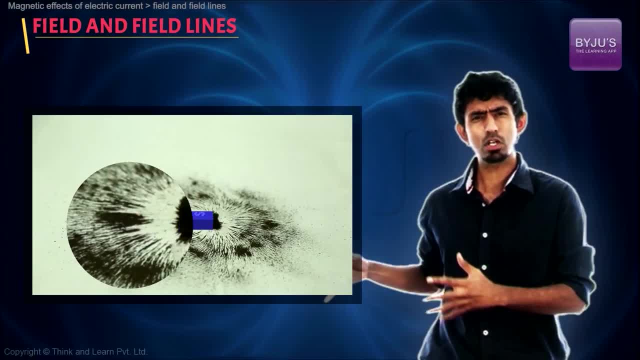 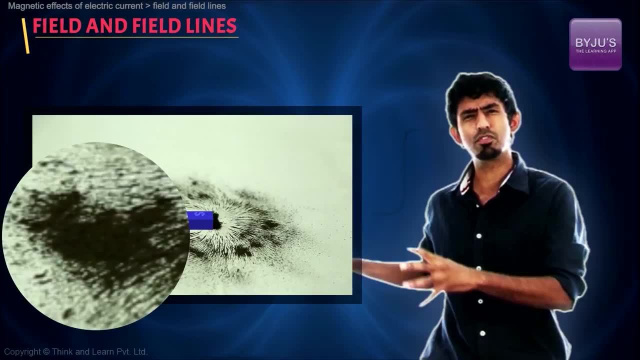 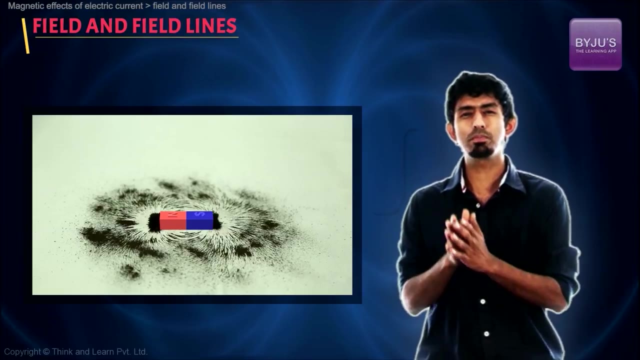 this happening. so if we go deeper into this we notice that somehow it looks like the area around this magnet is influenced by this magnet and you notice something: iron filings that are very far away are not really very affected. so we kind of realize this magnet's influence does not spread across forever, it stops or rather it becomes very, very